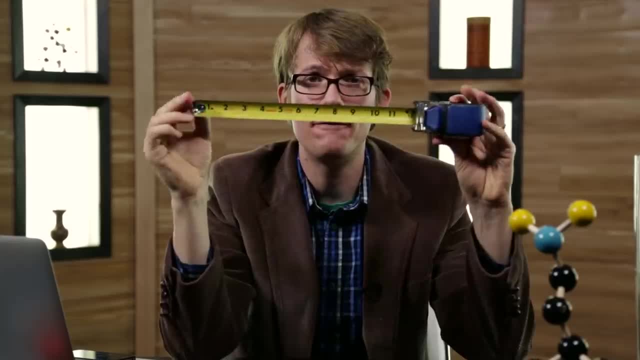 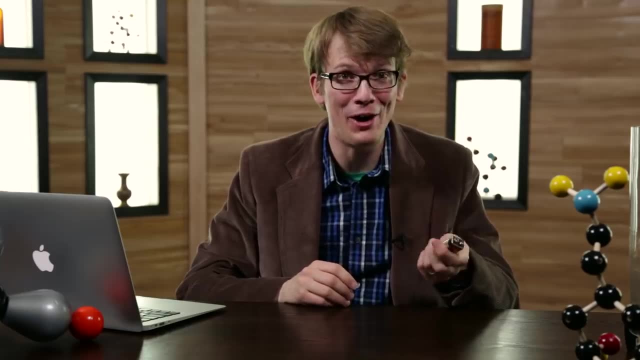 2,640 lumens, 1 foot, 2.3 kilograms, 9 volts. ah, I just closed the circuit with my tongue and I felt all 9 of the volts. So what do all these things have in common? They're units. 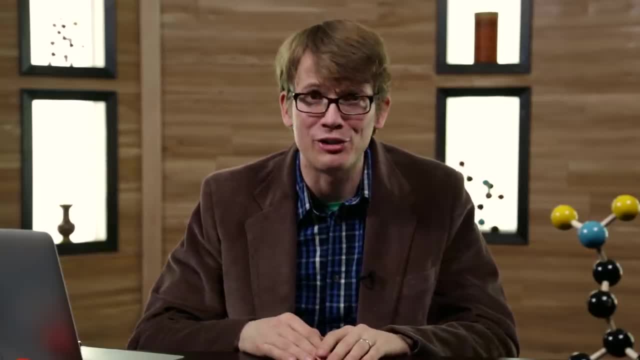 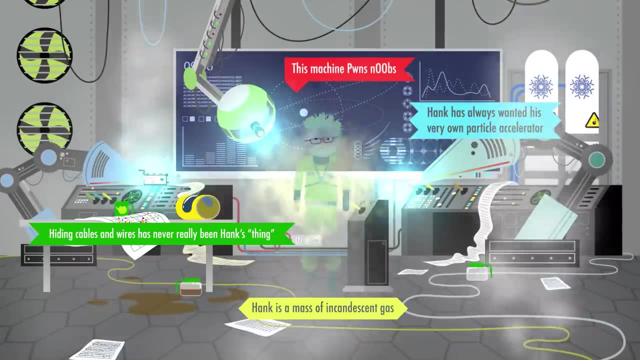 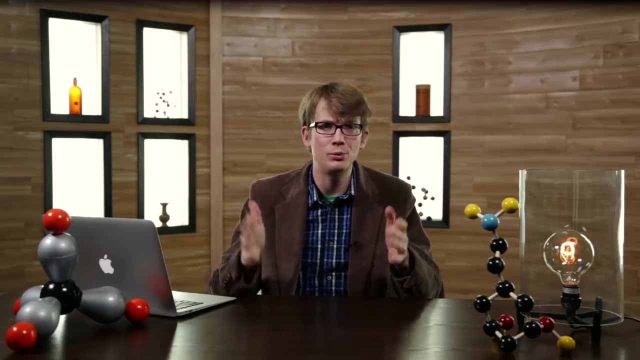 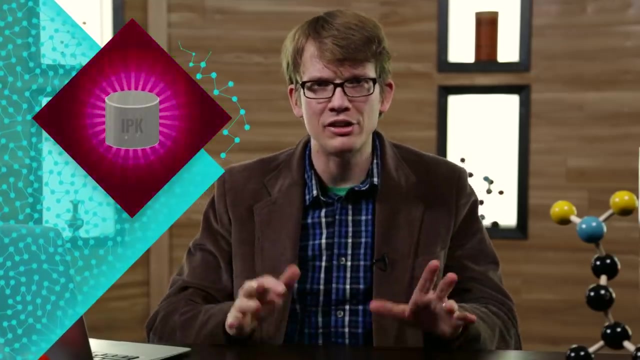 Yes, but they're also absolutely, completely arbitrary. You know who decides how much a kilogram weighs: A hunk of platinum and iridium known as the International Prototype Kilogram or IPK. The IPK isn't just how much a kilogram weighs. 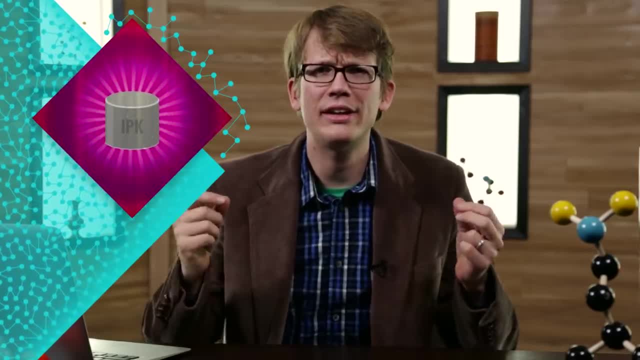 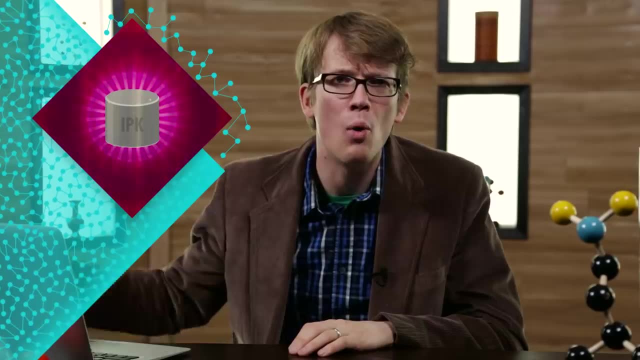 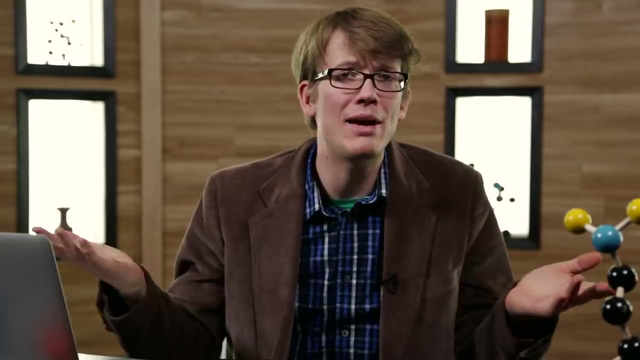 In a very real sense, the IPK is the kilogram. Every other kilogram is exactly the same as the IPK and the IPK is the lump of weight. It's the lump of metal that decides what that mass is. A kilogram is defined as being the same mass as the IPK. 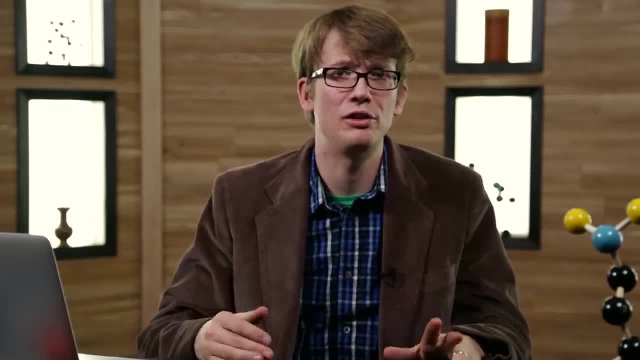 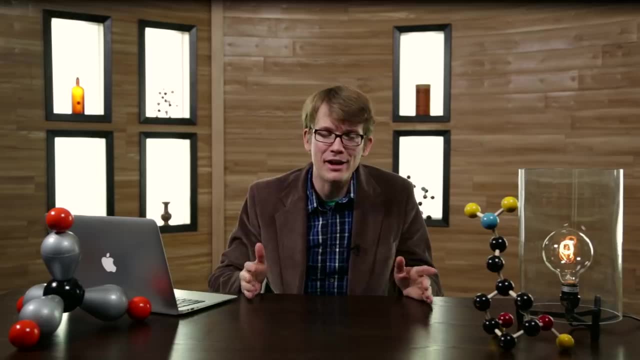 We made kilograms up, just like we made up seconds and weeks and volts and newtons. There's nothing about these things that makes them them. Someone just decided one day that that was a kilogram. Now, the fact that I find units fascinating probably says more about me than it does about 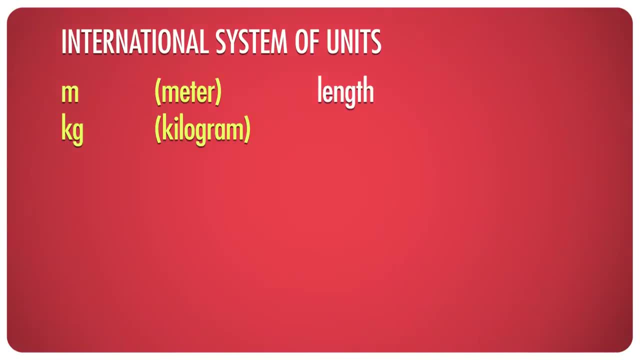 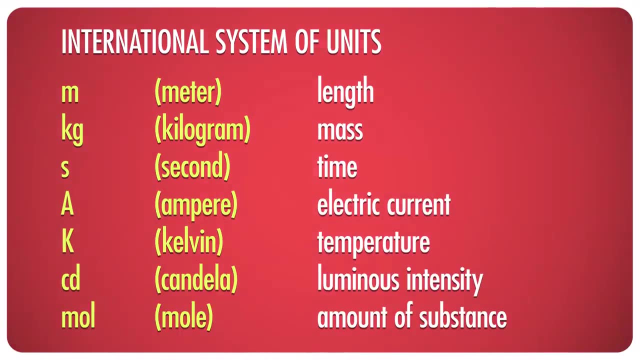 units, but I could talk about them all day. For example, did you know that the international system of units only includes seven base units And every other unit is derived from those units? Speed is length divided by time. Acceleration is speed divided by time, again. so meters per second, per second. 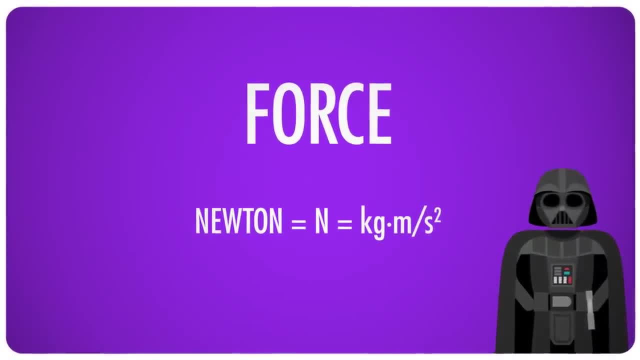 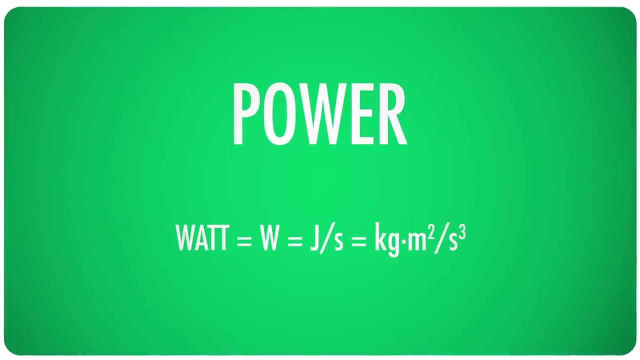 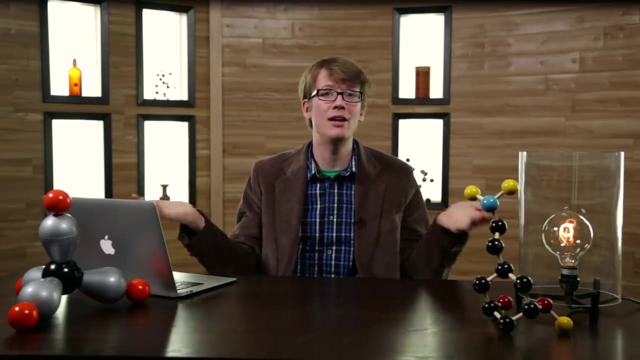 Force is that acceleration multiplied by mass, because F equals mA. remember Work done in joules is force multiplied by distance, And power is work divided by time. so how much work can be done per unit of time Makes sense. It goes pretty deep and it's absolutely correct to say that there are an infinite number of 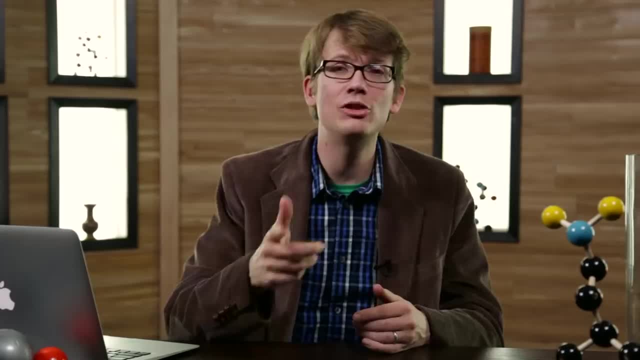 possible derived units. Just most of them are. Most of them aren't useful enough to name. But here's a bit of trivia for you. When I say watts or hertz, those things are just regular words, no special capitalization necessary. 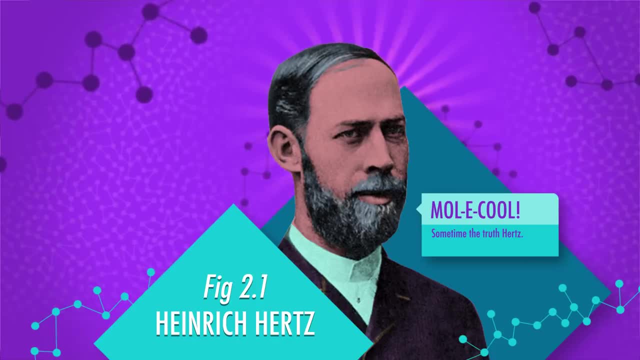 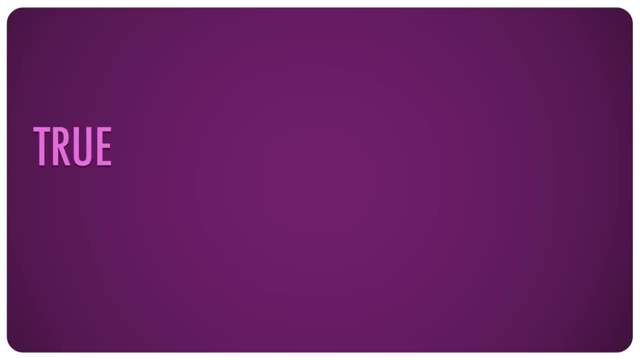 But hertz and watt, they were real people with, like last names that were capitalized. So what's up with that? Well, getting a unit named after you is kind of the holy grail of science, To quote Richard Hamming. true greatness is when your name, like hertz and watt, is spelled. 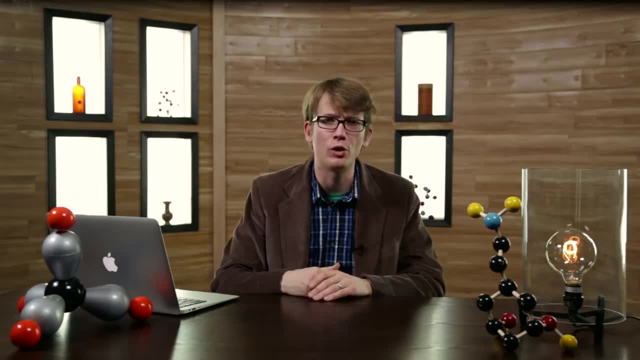 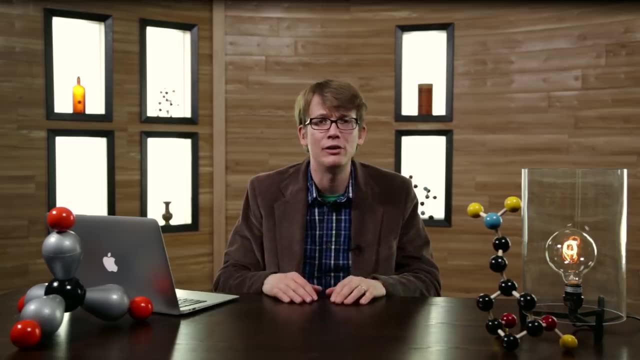 with a lowercase letter, Of course. when these geniuses were first piecing together how the world worked, they had no idea that there were fundamental basic units. They were basing all of their units on arbitrary values because, well, how could there possibly? 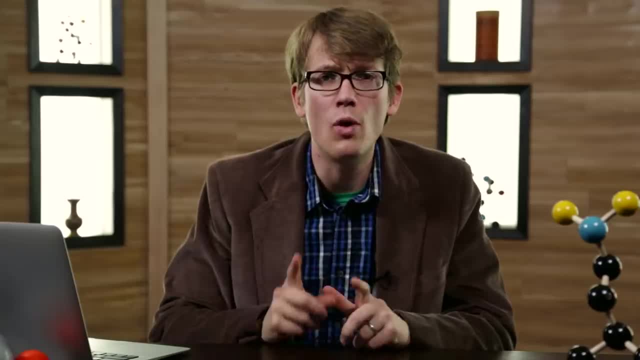 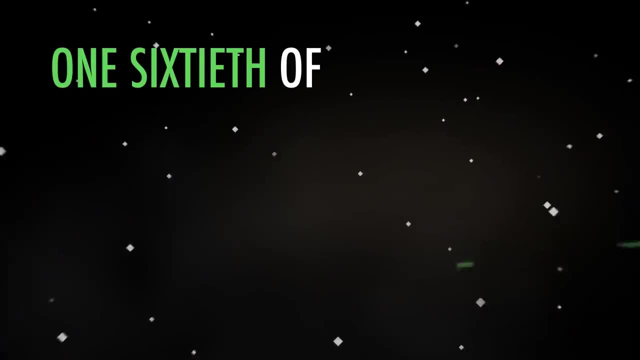 be a fundamental amount of mass or distance. Interestingly, one of the standard base units is derived from an actual value, though not a universal one. The second is one-sixtieth of one-sixtieth of one-twenty-fourth of the time it takes. 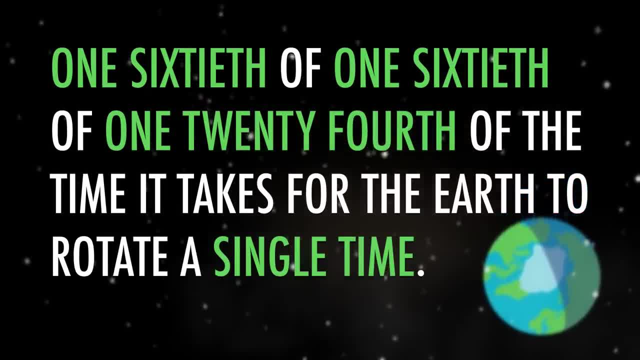 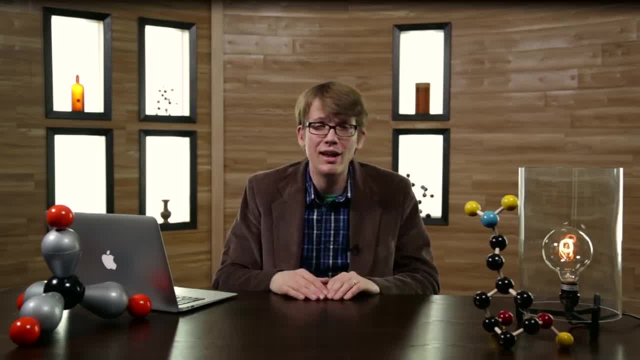 for the Earth to rotate a single time. That's something at least. but it also illustrates an interesting point. As fundamental as that seems, when you get down to the dirty details, things start to get kind of cloudy. The Earth's rotation, for example, is slowing down. Does that mean that seconds should also slow down? No, That would mess up every calculation ever so seconds are slowly becoming less and less based on reality. Now, don't worry, it's going to take forever for the Earth to slow down noticeably and 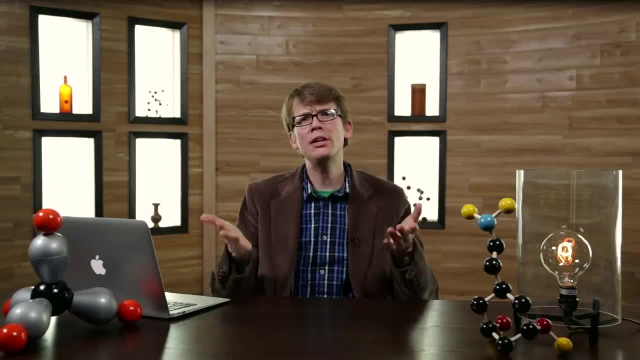 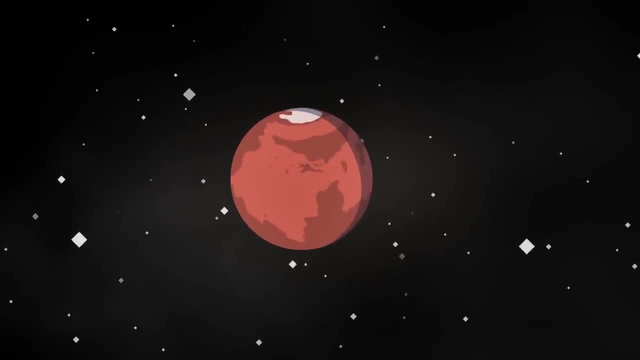 when it does, we'll just keep adding leap seconds to keep things balanced. But units are extremely important in chemistry and in sciences in general, as we learned when the Mars Climate Orbiter crashed into Mars because instructions were inputted in the wrong units. 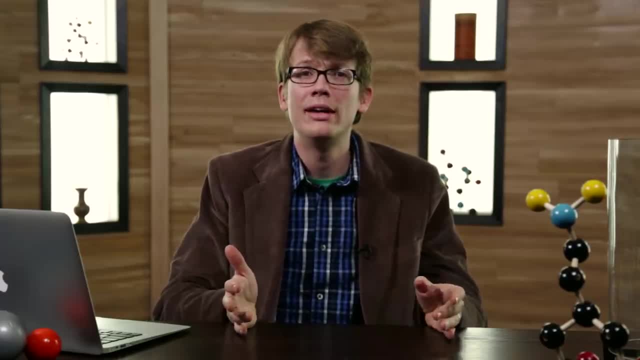 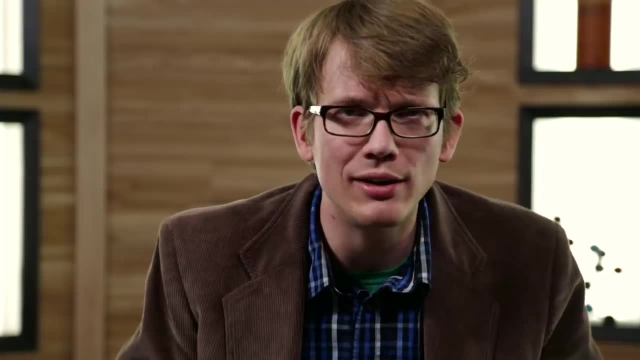 Sometimes you get a B instead of an A because you didn't keep track of your units. Just remember: at least you didn't destroy a 300 million dollar mission to Mars. But what do I mean when I say keep track of your units? 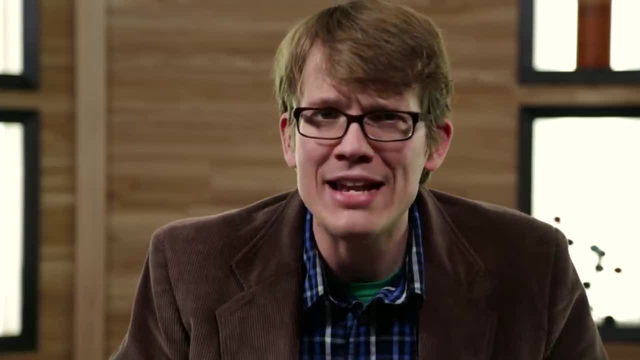 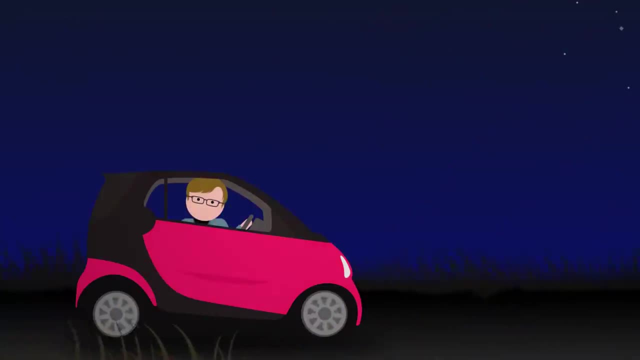 Well, I mean watch them. Do not let them do anything you didn't tell them to do, because they're sneaky and a lot of chemistry is just converting between units. So say, you're in a car and the car is going 60 miles per hour. 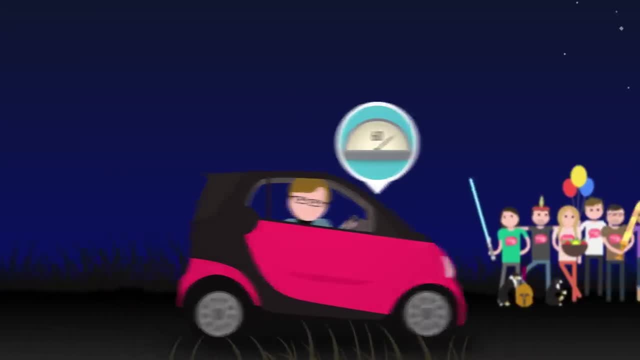 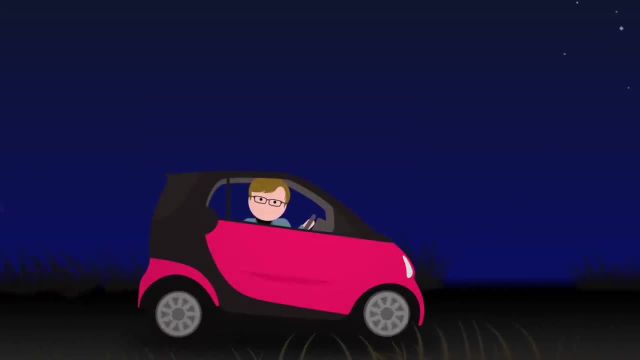 Now, right now, everyone who doesn't live in America is like boo. miles are terrible, convert to kilometers. Well, I'll do you one better. From a scientific perspective, kilometers are terrible too. They're just as arbitrary. We should use something more universal, like light years, the amount of distance light. 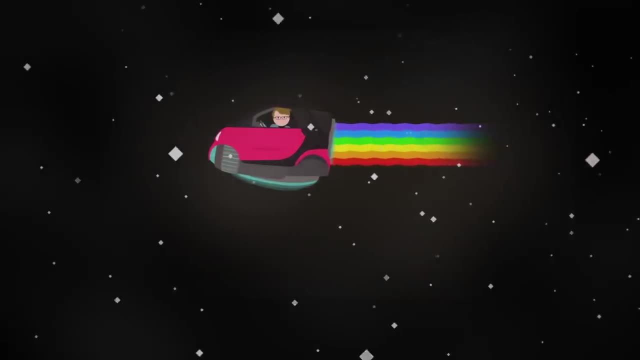 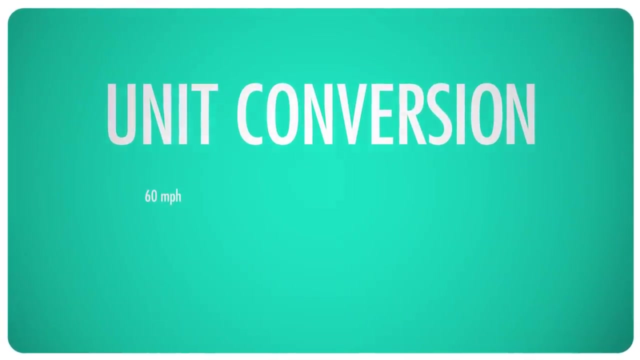 can travel in a year, And hours, hours is no fun, so let's convert to light. years per second. 60 miles per hour: When you say it, it sounds like a whole number with a single unit, but it's not. 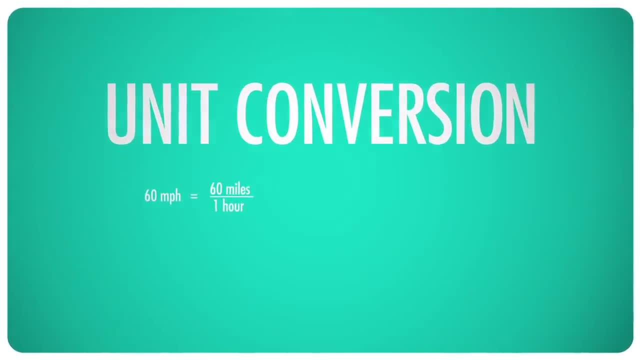 It's actually a fraction: 60 miles over one hour. Let's start with the easy part, getting to seconds. So first we've got to get to minutes. So there's 60 minutes per hour And also one hour per 60 minutes. 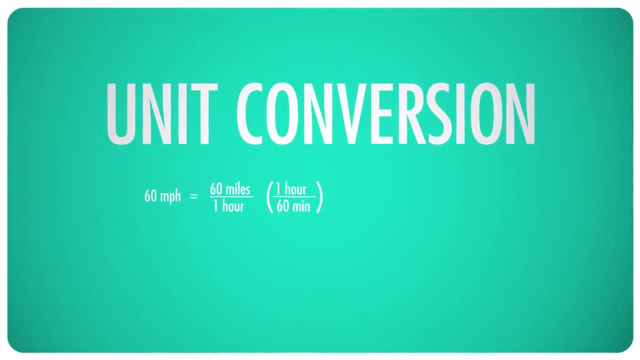 That fraction, once we have it can flip either way. We want it with the hours on the top on the numerator. Why? Because we want the units to cancel. We want to destroy the hours. We don't want them in our units when we're done. 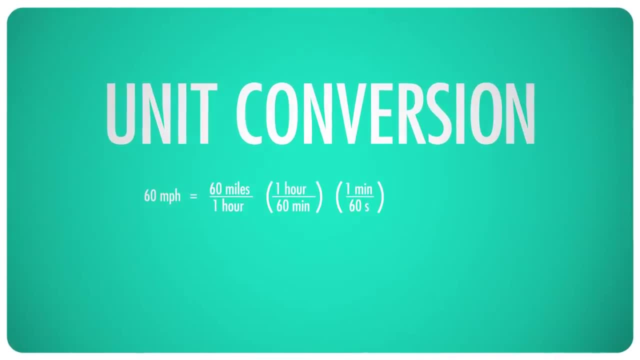 Then the same thing happens again with one minute per 60 seconds. Now we go to light years. I asked Google and there's one light year in every 5.9 times 10 to the 12th miles. Looking at this, we see that the hours cancel and the minutes cancel and the miles cancel. 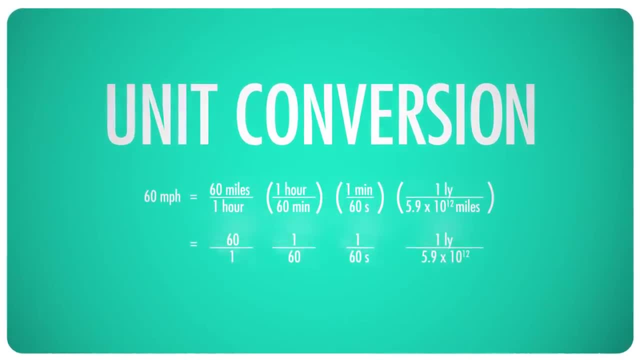 leaving us with light years per second. That's really what matters. We've come out with the correct units. The rest is just hammering at the calculator to discover that a car going 60 miles per hour is also going 9.3 times 10 to the negative 12th light years per second. 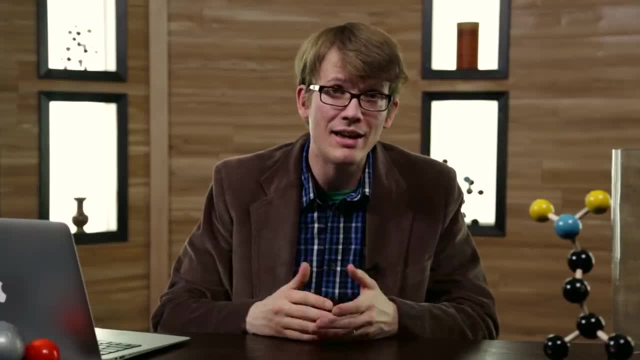 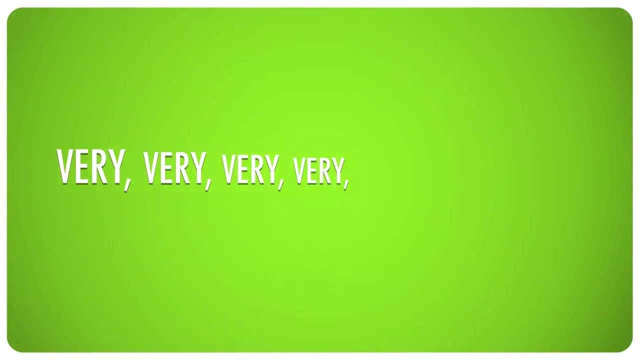 Now we perform an important test, the does this make sense test? And, yes, indeed it does, because 9.3 times 10 to the negative 12th is a very, very, very, very small number, which makes sense because when you're traveling in a car, you're going. 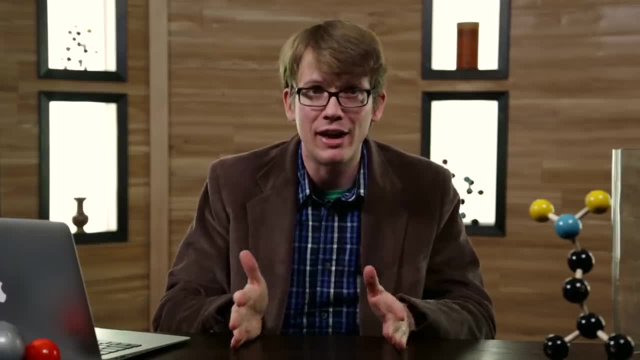 a very, very, very, very, very, very, very tiny fraction of a light year per second. That's really what matters. We've come out with the correct units. We've come out with the correct units. We've come out with the right units. 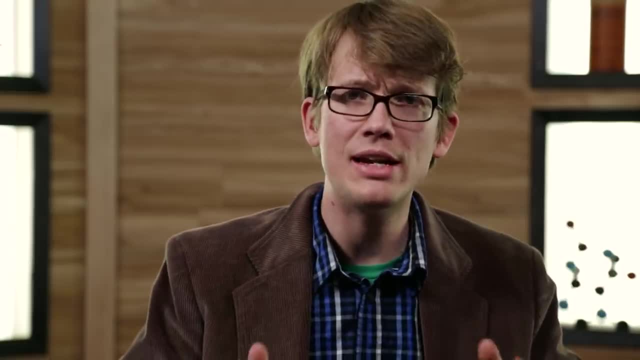 We've come out with the correct units. We've come out with the correct units And we've come out with the correct units And we've come out with the correct units. Now there are probably gonna be 50 to 100,000 people that watch this video, and I'm gonna 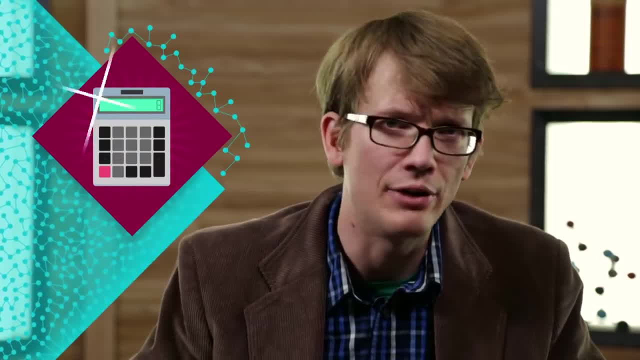 guess that maybe a solid seven of you did the math along with me with your calculator out. Now I'm not giving you a hard time. that is just my guess. If you want to follow along with your calculator in the future, that might be helpful. 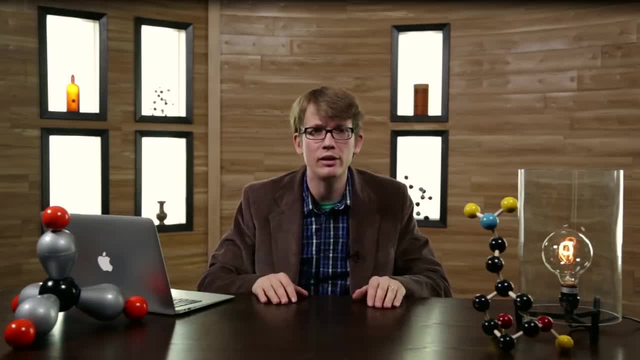 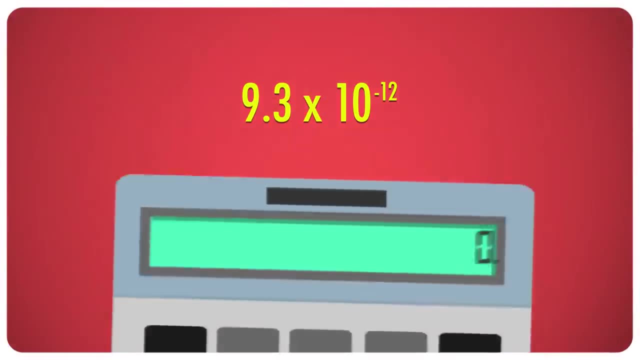 It would at the very least be very nerdy. But if you have been following along with your calculator you might maybe have noticed something interesting. I said 9.3 times 10 to the negative 12th, when your calculator, your calculator, probably. 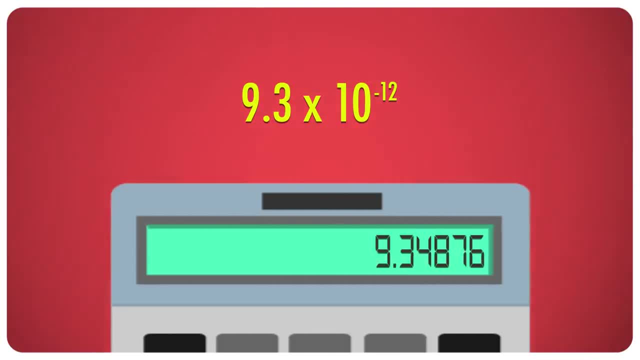 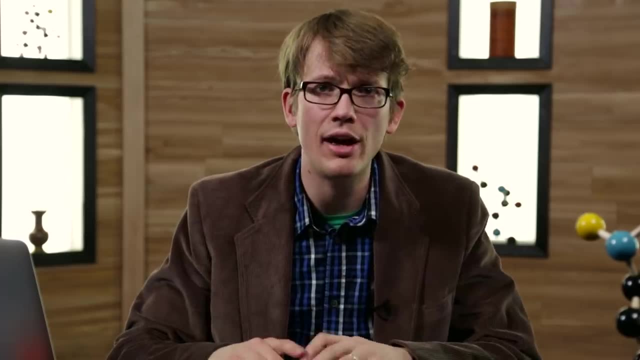 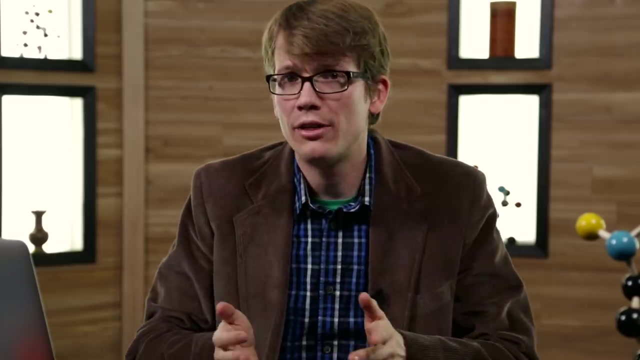 said something like 9.9.. So why, when I had so many more numbers to give, did I only give two? Was I trying to save time? Well, obviously not, because now I appear to be wasting time talking about it. 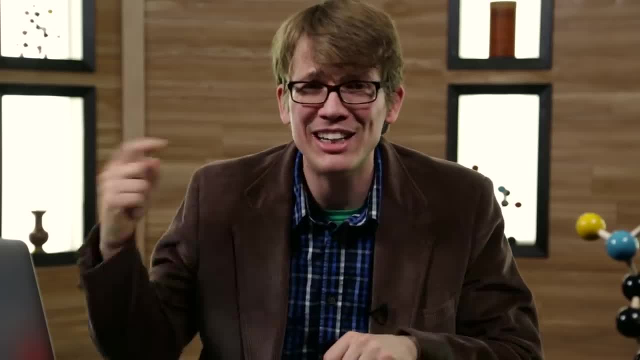 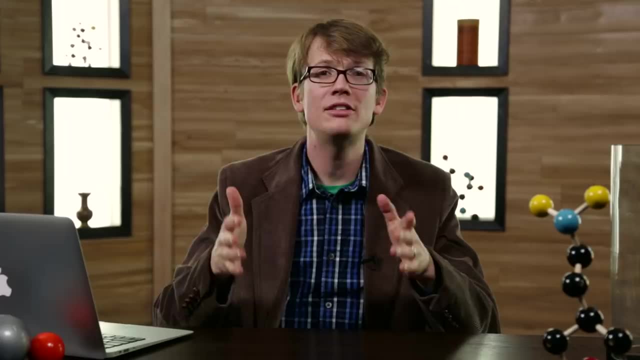 Do you think that it would be too hard for me to remember all those numbers? Well, obviously not, because I just did it. So I will tell you why. When you're doing experimental calculations, there's two kinds of numbers: There's exact and measured. 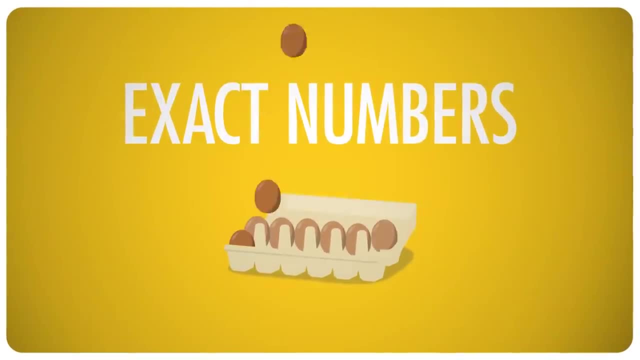 Exact numbers are like the number of seconds in a minute or the number of eggs in a dozen. They're defined that way, and thus we know them, in effect, all the way out to an infinite number of decimal places. If I say that there are a dozen eggs, you know that that's 12.. 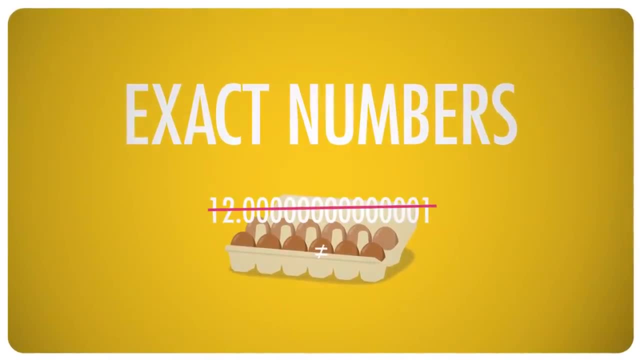 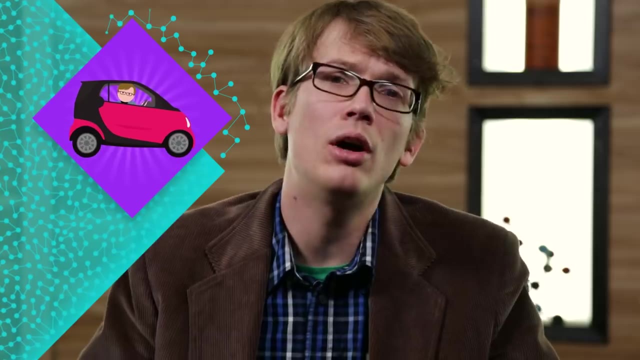 It's not 12.000000001, or 11.999999.. It's 12.. But that's not true for the number of miles per hour my car was going. That car wasn't going 60.0000 out into infinity miles per hour. 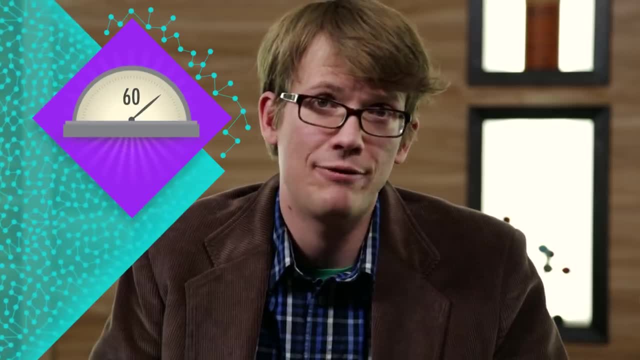 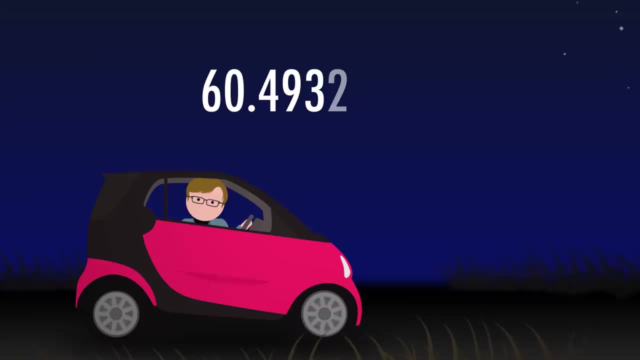 I only know the speed of my car. I only know the speed of my car to two decimal places, because that's all I get from the speedometer. So the car could have been going 59.87390039 miles per hour or 60.49321289 miles per hour. 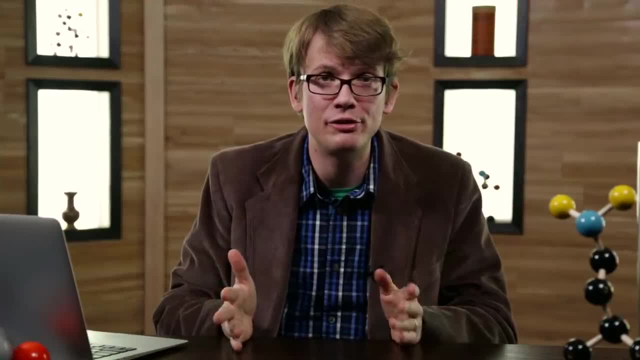 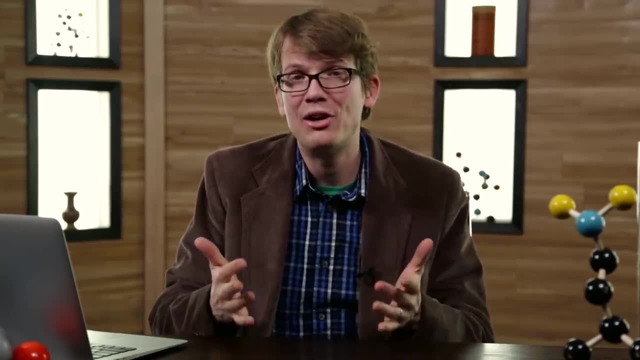 The speedometer would still say 60. And no matter how well I measure the car's speed, I will never know it at the same level of precision that I know the number of eggs in a dozen. So that's the second type of number, measured numbers. 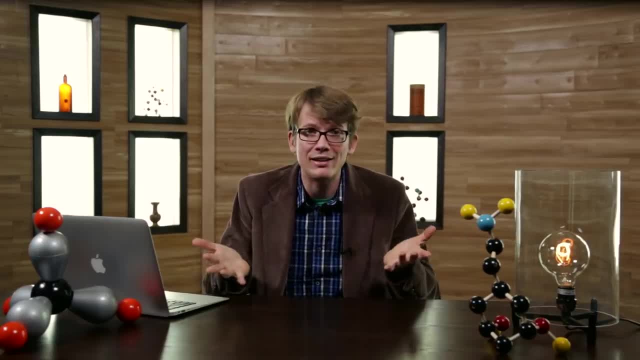 Now, the cool thing about measured numbers- because you never, ever know them exactly- is that they tell you two things at once: First, they tell you the number that you're going to measure, And then they tell you the number that you're going to measure. 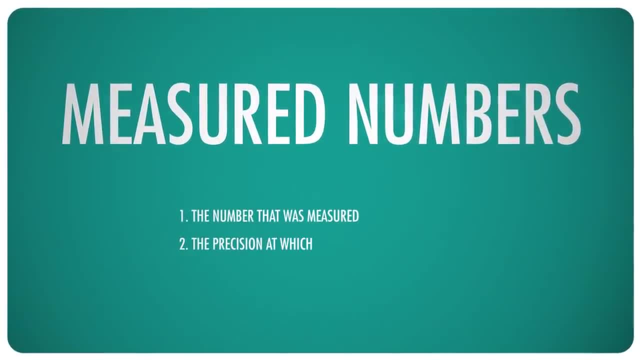 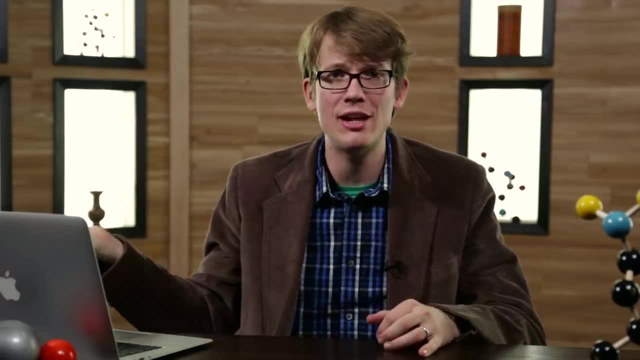 And then they tell you the number that you're going to measure And second, they tell you the precision at which that number was measured. People often get their heads all tangled up about this, but with a measured number, you just have to remember that the actual number goes out to infinite decimal places. 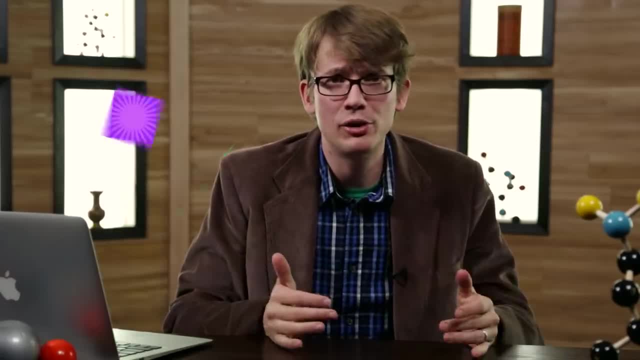 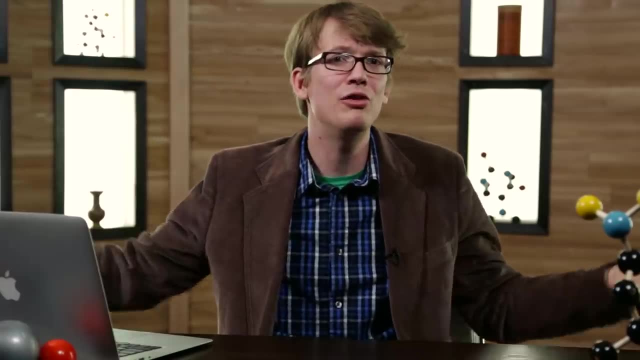 You just never know all of them. You can't, It's impossible. So when my scale says 175 pounds, that doesn't mean 175.000000 pounds, It means 175 point something pounds And all those numbers after the five. We don't know them. And here's the thing: A measured number can be pretty unhelpful if you don't have knowledge of the precision of the measurement. So you have to conserve the precision through your calculations, or else you might end up. 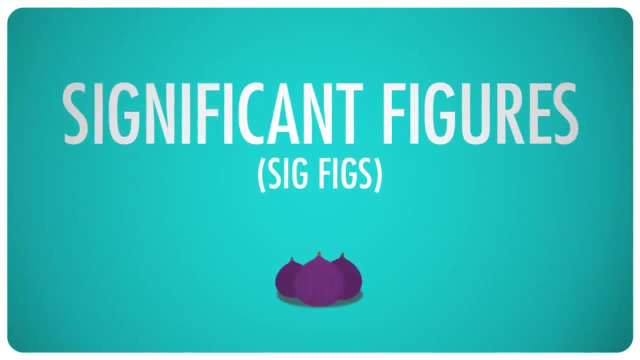 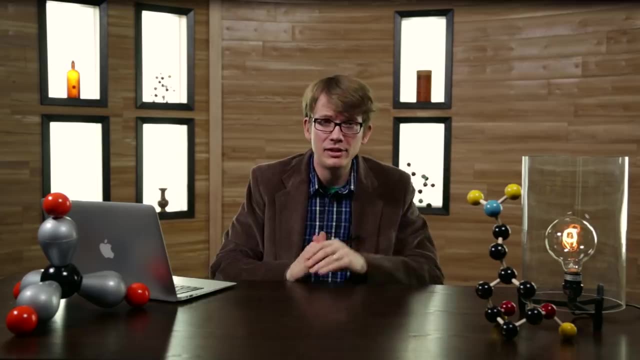 killing someone with an imprecise dose of insulin or something. So we have a set of rules for what are called significant figures. These are the digits in your number that you actually know With my speedometer. there are two, six and zero. 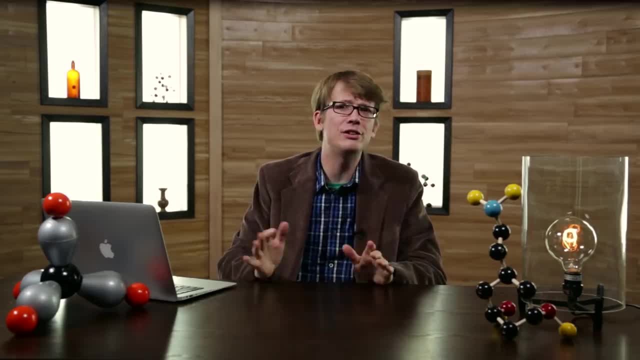 But zero is weird because sometimes it's just used as a placeholder, Like if I said that the fastest plane can go 13,000 miles per hour, which it can, by the way, An unmanned military test glider did it in 2012.. 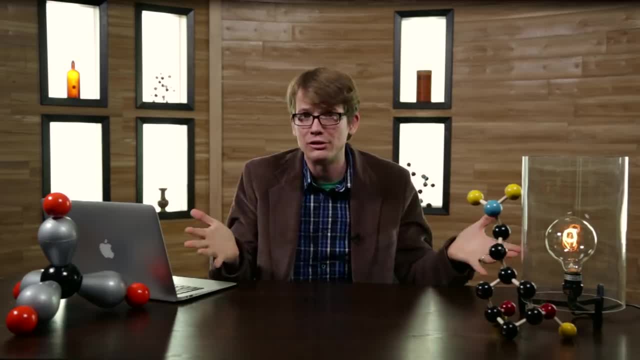 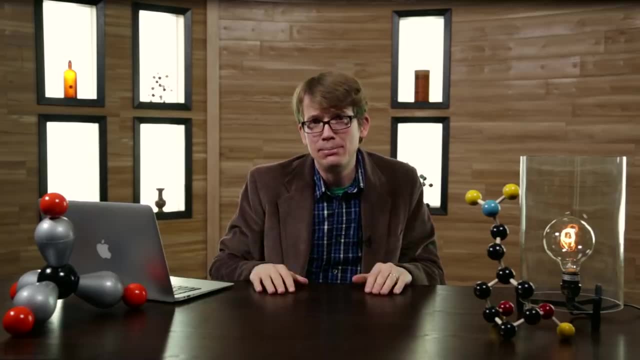 In 2011,. that's not an exact number. Those zeros are just placeholders, So when a number ends in a zero, or two or three zeros, it's hard to tell if those zeros are significant. But this all gets so much simpler when you use scientific notation which, since it's 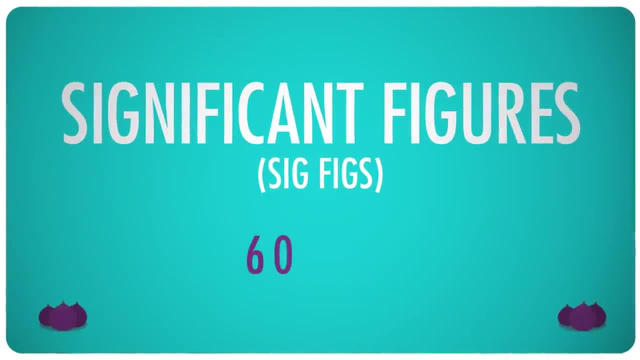 science we should. So 60 miles per hour would instead be 6.0 times 10 to the first power We get. that zero is significant because we wrote it, Otherwise it would just be 6 times 10 to the first power. 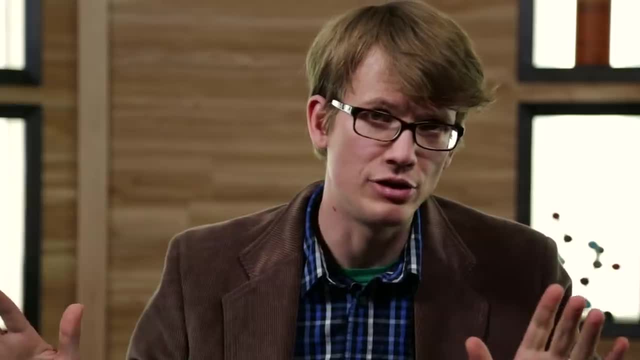 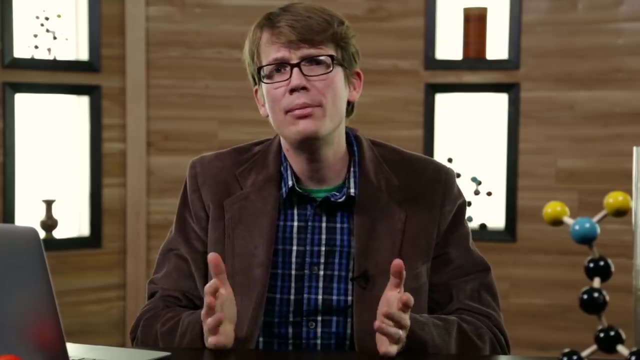 We keep that zero around because we actually know it. Scientific notation is awesome, by the way, Once you get the hang of it. If you're having trouble, you can always just type it into Google or your calculator to see exactly what number we're talking about. 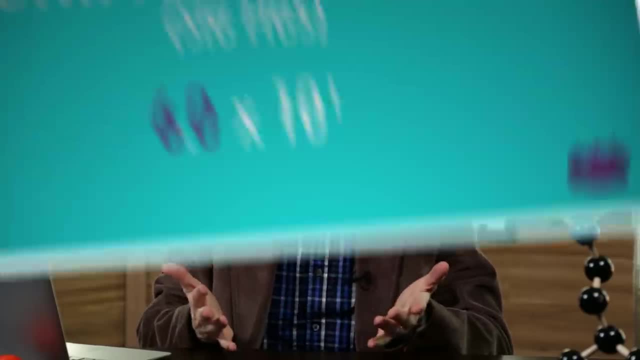 But the number of the exponent just tells you how many places to move the decimal point. So to the first power: you move it one to the right and you get 60.. To the negative first power: you move the decimal point one place to the left and you. 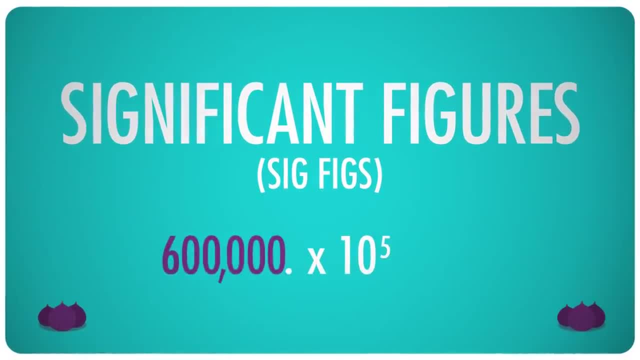 get 0.60.. To the fifth power: 1,, 2,, 3,, 4,, 5, and you get 6 with five zeros, or 600,000.. Of course, your significant figures get preserved. so 2.4590 times 10. to the negative fourth: 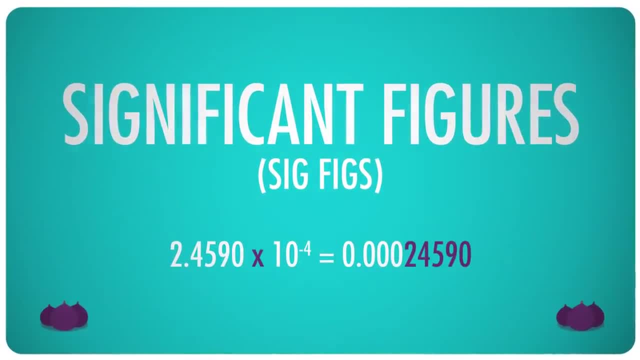 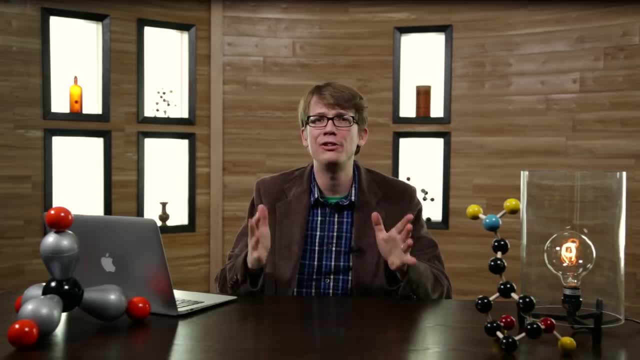 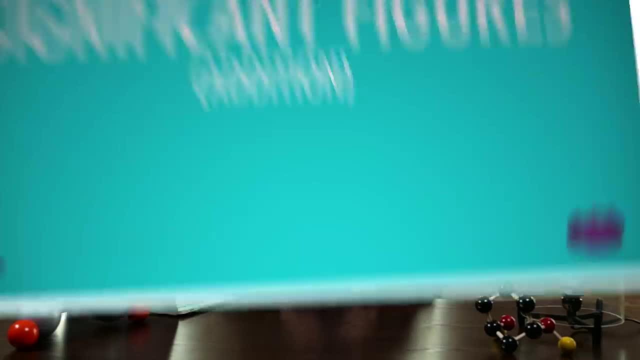 There are two simple rules for this. If it's addition or subtraction, it's only the number of figures after the decimal point that matters. The number with the fewest figures after the decimal point decides how many figures you can have after the decimal in your answer. 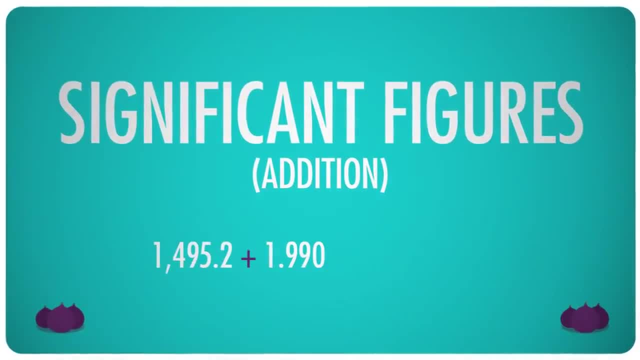 So 1,495.2 plus 1.9903.. You do the math: first You get 1,497.1903, and then you round to the first decimal, because that first number only had one figure after the decimal. so you get 1,497.2.. 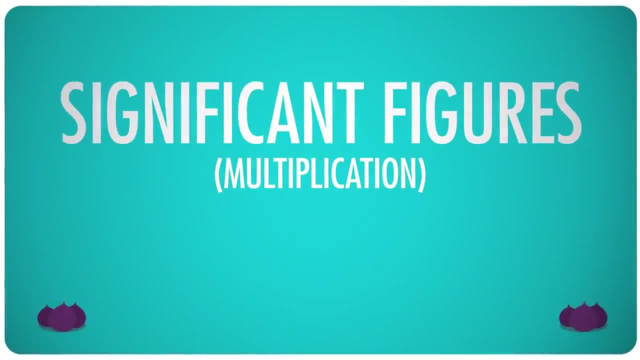 And for multiplication, just make sure your answer has the same number of sig figs as your least precise measurement. So 60 times 5.0839 is 305.034, but we only know two sig figs, so everything after those. 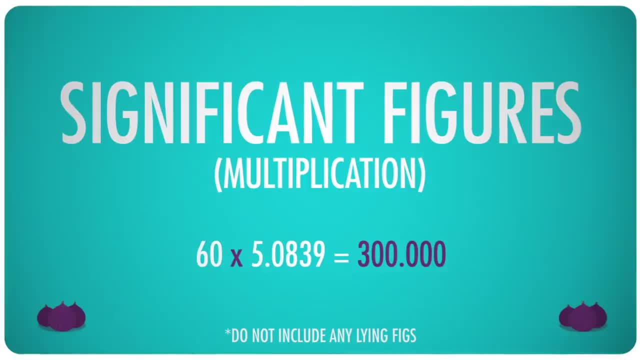 first two numbers is zeros 300.. Of course, then we'd have to point out to everyone that the second zero, but not the third, is significant. so we'd write it out with scientific notation: 3.0 times 10 to. 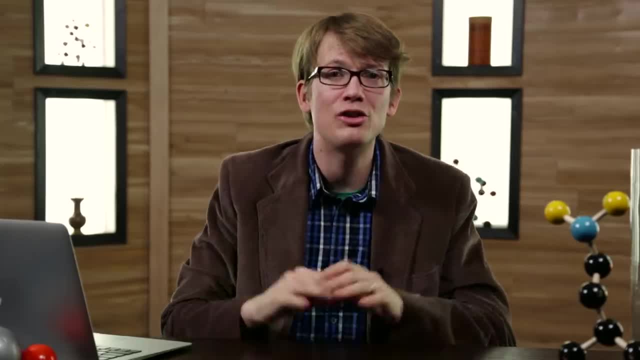 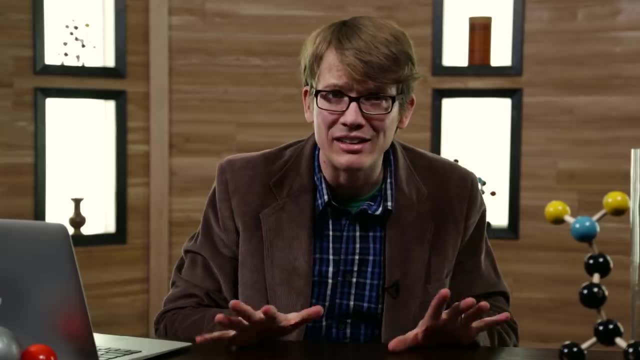 the second power Because science. Now, I know it feels counterintuitive not to show all of the numbers that you have at your fingertips, but you gotta realize all of those numbers, beyond the number of sig figs you have, they're lies. 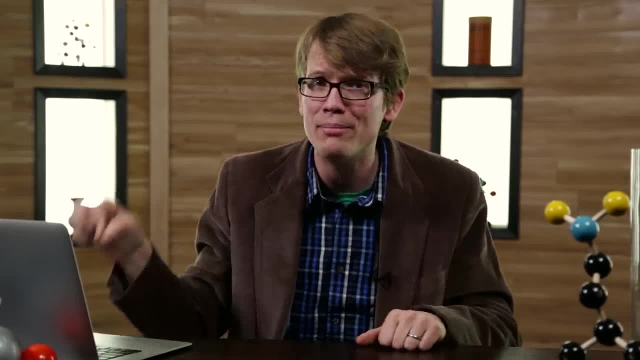 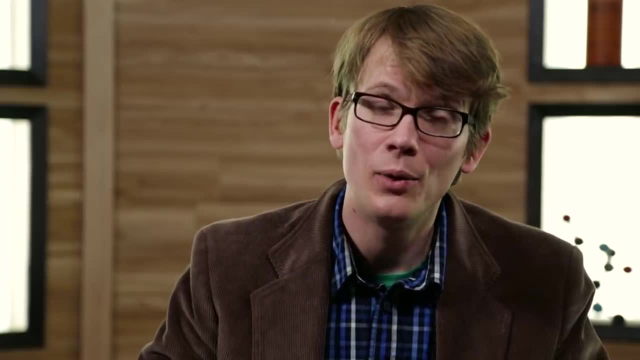 They're big lying numbers. You don't know those numbers and if you write them down, people will assume that you do know those numbers and you will have lied to them. And do you know what we do with liars in chemistry?